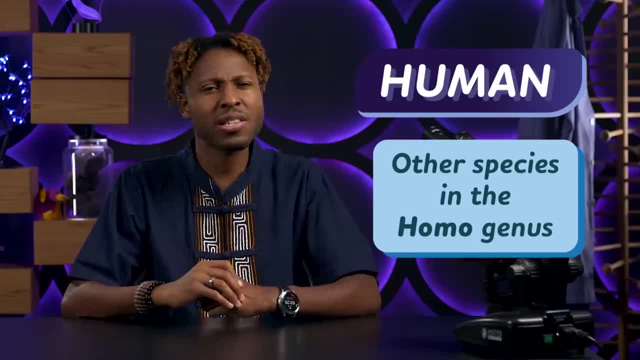 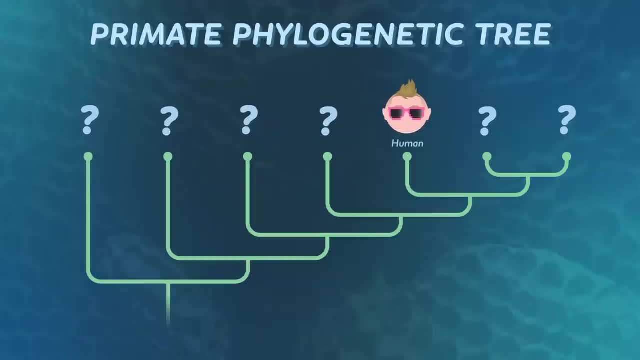 including those close relatives that we share the planet with, Which leaves us with the burning question: What is a human Well? for starters, all our closest kin have been extinct for at least the last 40,000 years, So today we humans have more in common with chimpanzees and bonobos. 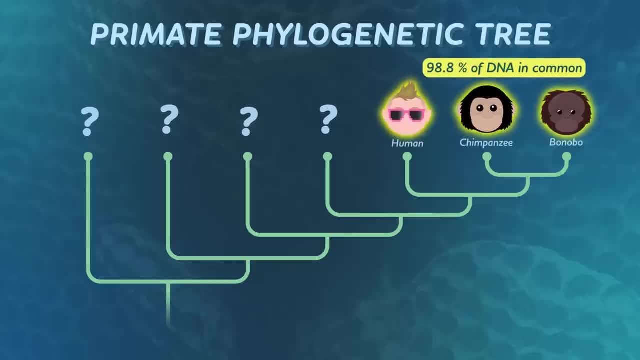 than any other living species. We share about 99% of our DNA with them. In fact, chimps are more closely related to us than they are to their gorilla cousins. Humans and chimps are both members of our DNA. We're all members of the large primate group which includes our distant cousins. 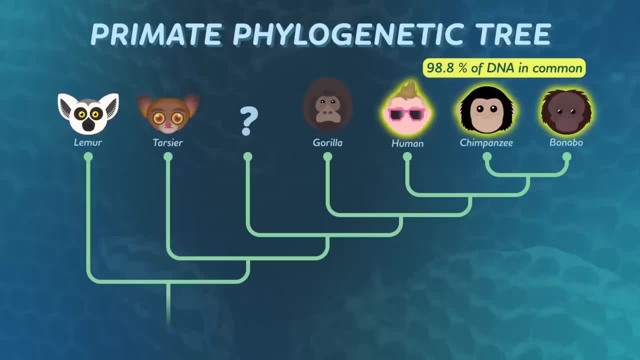 like lemurs and tarsiers, And also some not-so-quite-distant ones like gorillas and orangutans, But humans didn't evolve from chimps, Or any other living ape for that matter. Chimps and humans split from a common primate ancestor around 7 million years ago. 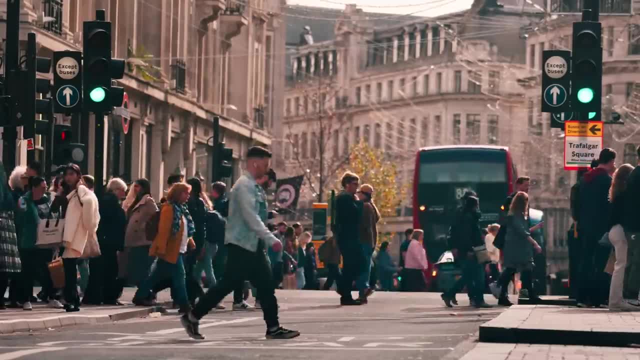 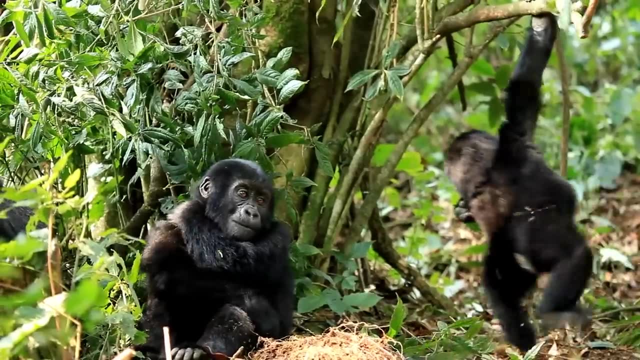 And we've each been moving along our own evolutionary branches ever since then, Alongside many other branching species, some that survive to today and many that didn't. So yeah, there's no straight line. There's no straight line from chimps to humans. 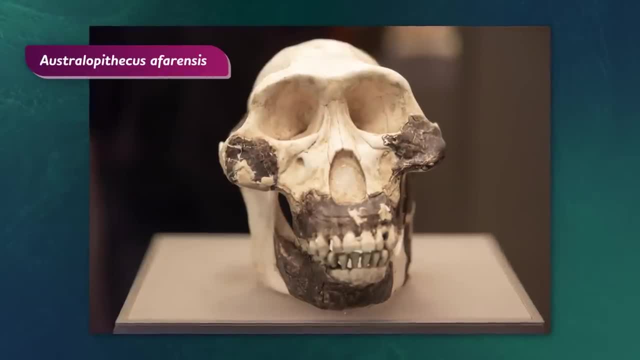 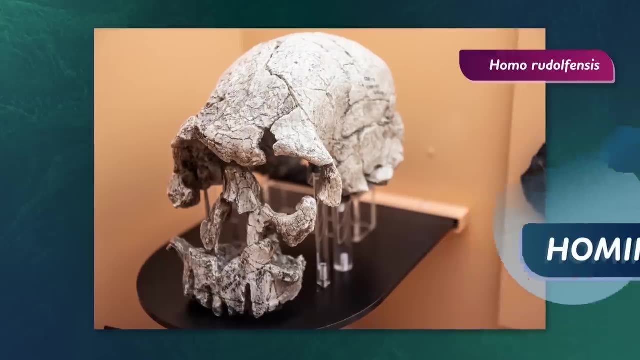 But there are a lot of branching ones And there's still a lot that we don't fully understand about our branch, the hominins. We know of at least 20 other hominin species from fossil and DNA evidence that have lived across the past 7 million years. 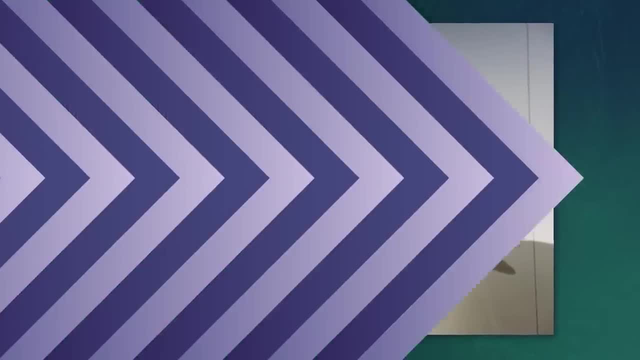 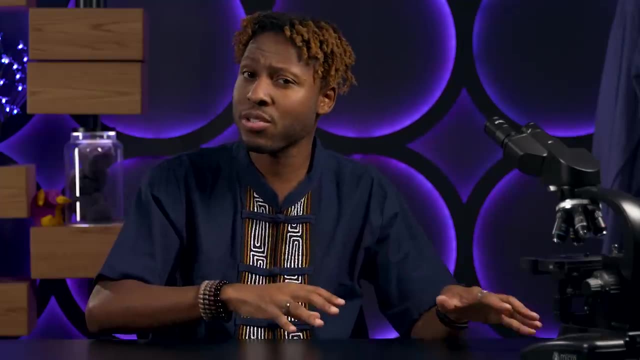 But we're still working out how those hominins are related to each other and to us, Like they're all your relatives But they're not all your ancestors. They didn't descend from your grandma's sister, but she's still part of your family. 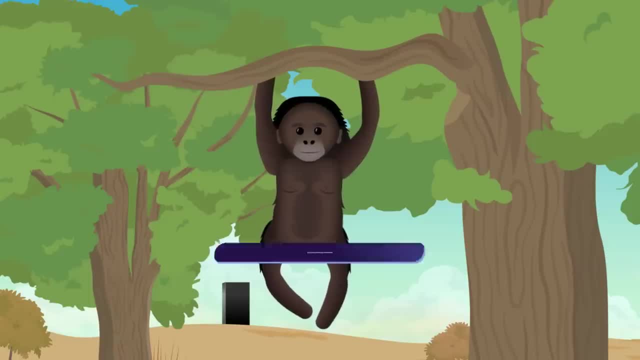 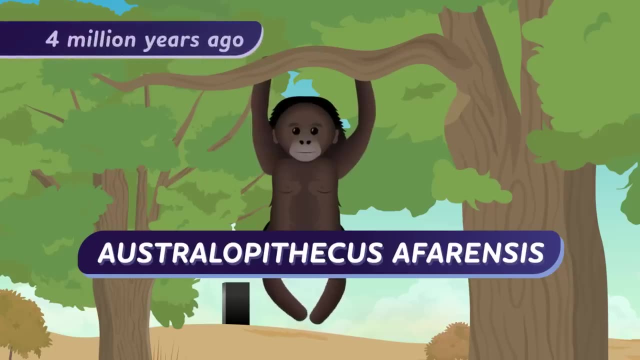 Love you, Great-Auntie. We do have a good hunch that one of those fellow hominins, Australopithecus afarensis, was basically humanity's grandma. Little afarensis lived about 4 million years ago in Africa. 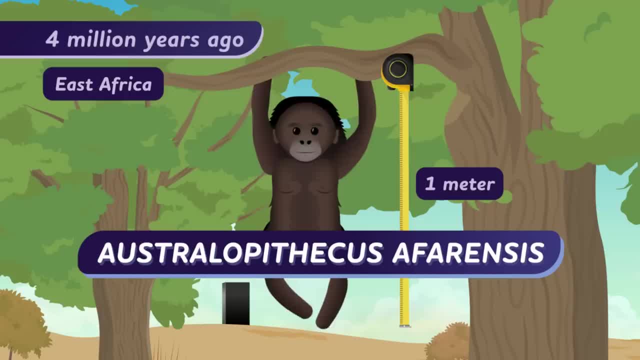 They were only 1 meter tall, with arms longer than their legs and a small brain, And, based on the clues from fossilized hips, skulls and footprints, we think afarensis did something that at the time, was a little odd for apes. 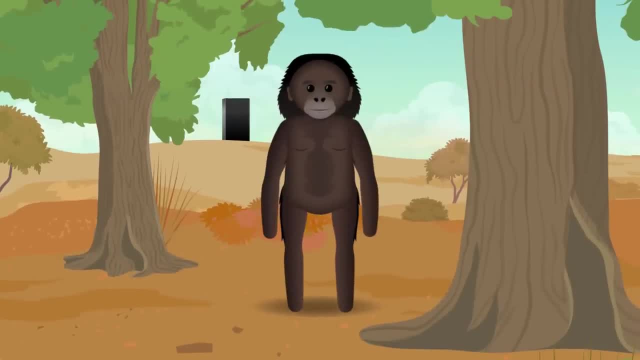 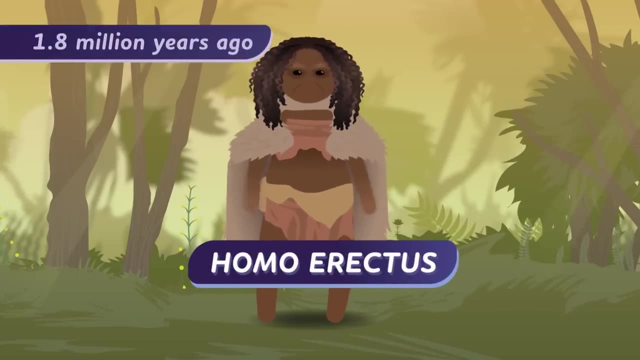 But has since become pretty rare. Some pretty commonplace for humans Walk around on two legs. Another likely human ancestor, Homo erectus, strutted their stuff starting around 1.8 million years ago. They had a head about twice the size of afarensis', with body proportions roughly equivalent to. 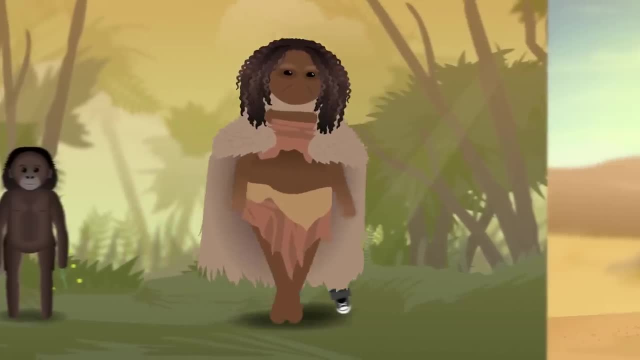 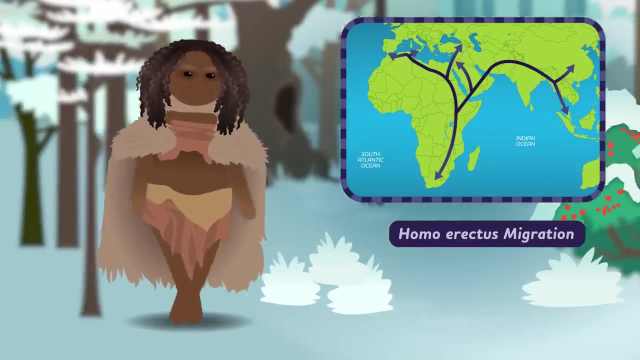 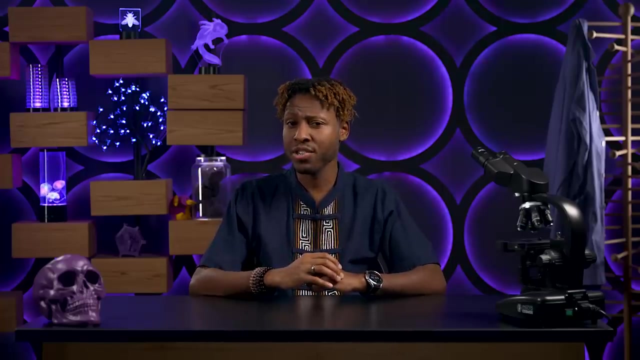 modern humans, great for long-distance walking. In fact, they were the first hominin to make the long trek out of Africa and hang out in Europe and Asia, Kind of like the original gap year backpackers. While these two ancient ancestors shed some light on how early humans lived, most of our relationships with other hominins remain. 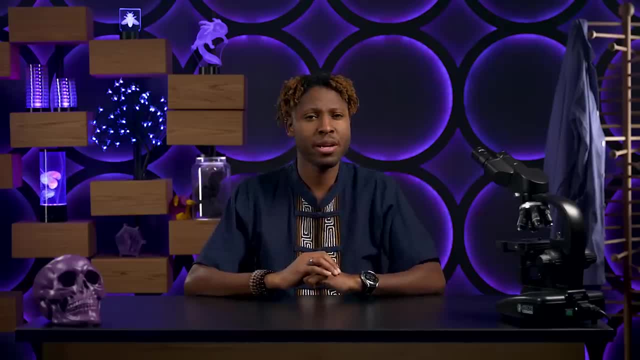 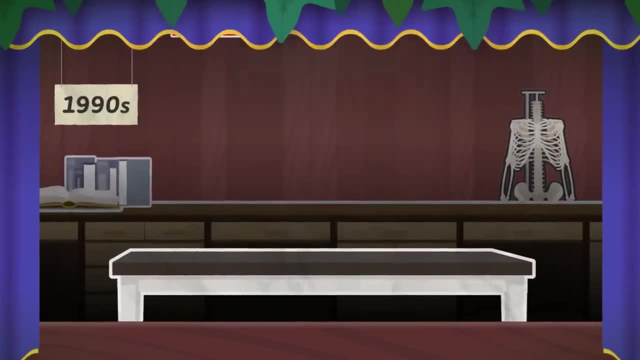 murky and debated. The more we learn about the hominin family tree, the more we realize it might not be much of a tree at all. Let's take a trip to the theater of life In the 1990s, the Chinese paleontologist Dr Zhin-Chi Wu, 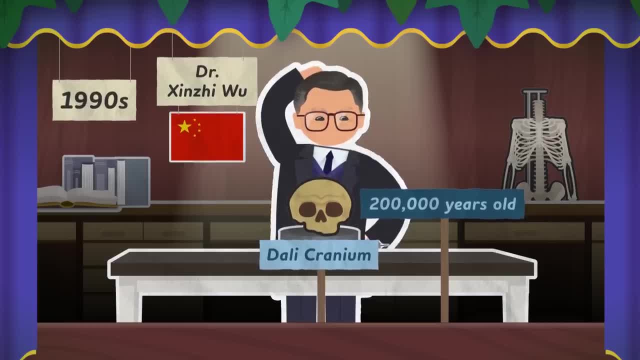 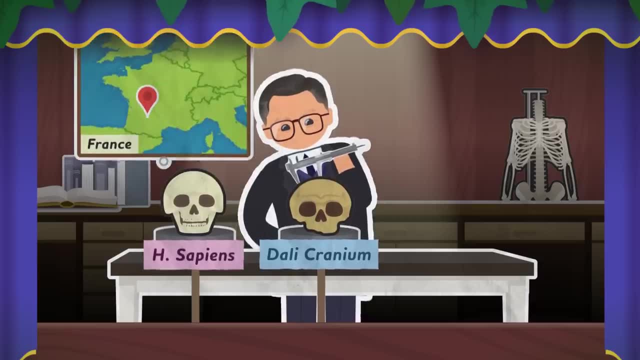 found himself puzzled over a 200,000-year-old skull called the Ta-Li cranium, Thick and heavy-browed with a medium-sized brain. in some ways it looked like Homo sapiens fossils from Europe, But in other ways it resembled fossils of Homo erectus from China. 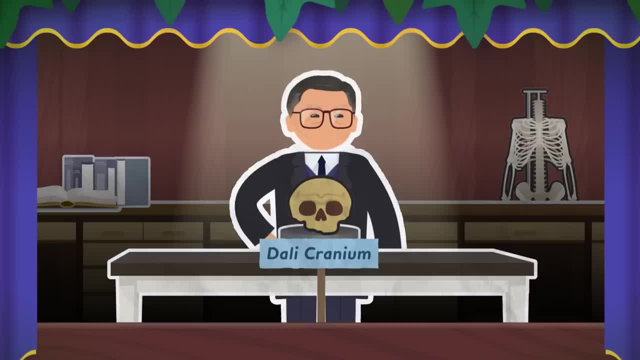 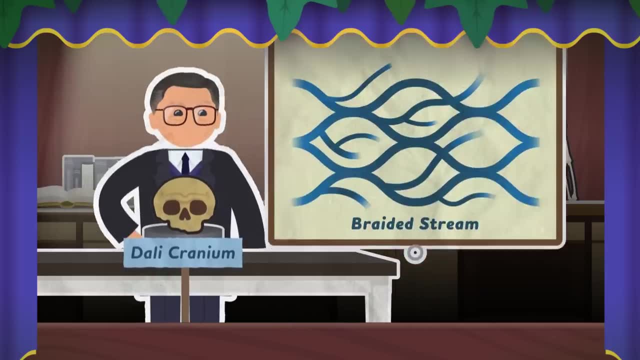 Basically, it was a real mixed bag. So Dr Wu came up with the hypothesis: What if this species wasn't just another branch of the evolutionary tree? What if, instead, this was a sign of evolution working like a braided stream, with populations sometimes trickling and drifting away? 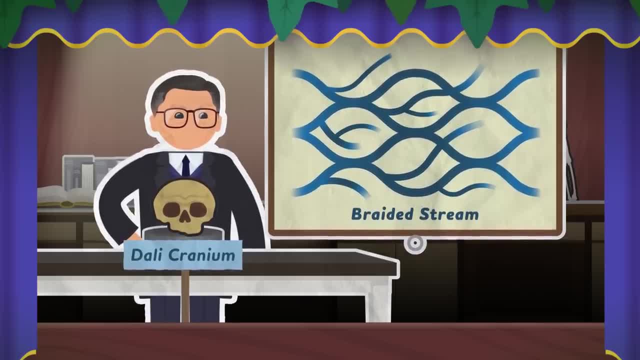 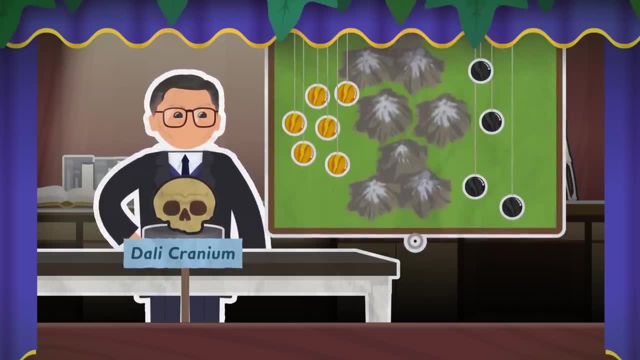 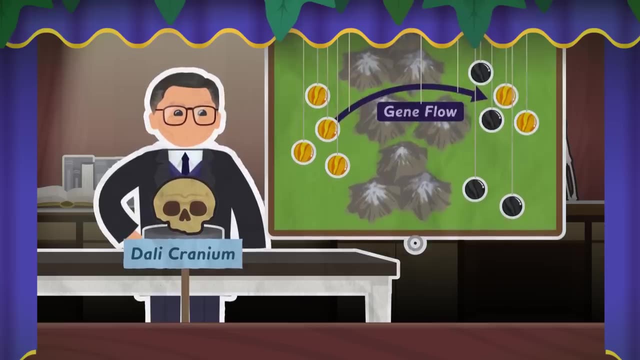 but then eventually merging back again into the same flow. He imagined a pattern like this: When populations become isolated for generations, which means not reproducing without outsiders- they become different and evolve distinct traits, But sometimes those populations link back up and swap genes again. 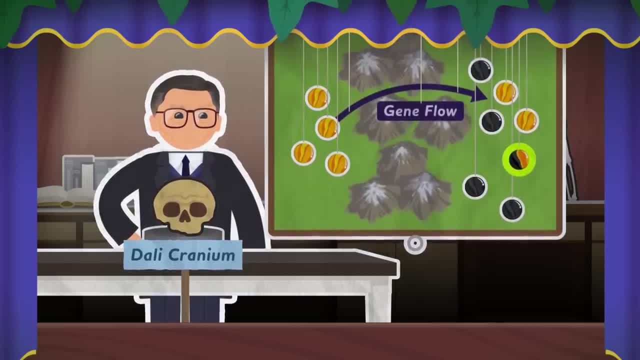 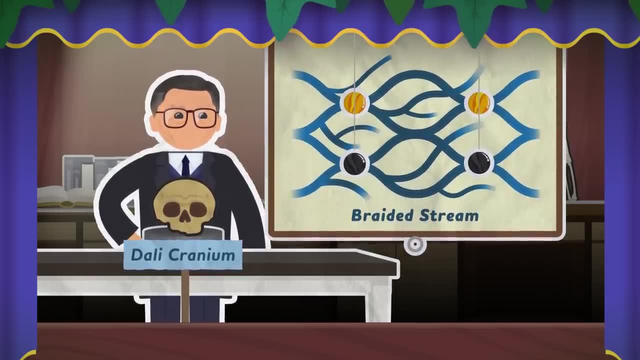 and those genetic differences start to give way to similarities once more. With these ebbs and flows, populations alternate between times where they're apart, drifting on their own course, and times where they're connected with a steady flow of genes between them. 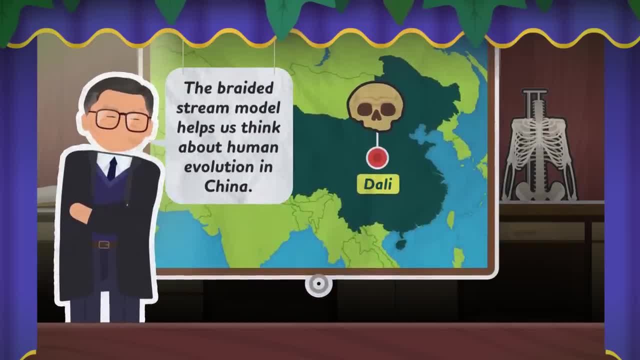 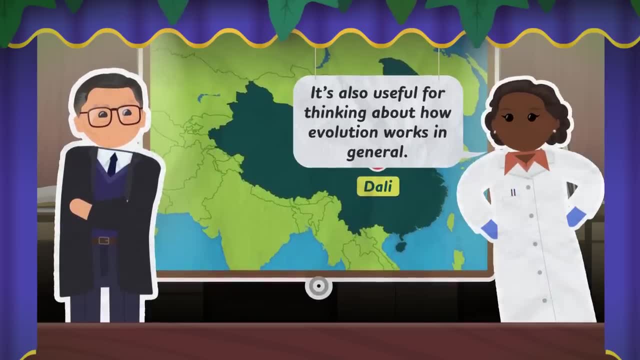 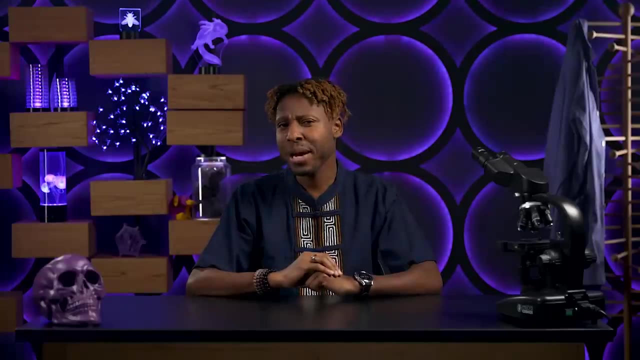 Dr Wu originally used the braided stream analogy to think about how human evolution played out in China, But today many scientists agree it's a useful model for thinking about how humans evolved across the planet and how evolution works in general. With better technology, scientists have been able to extract ancient DNA from fossils. 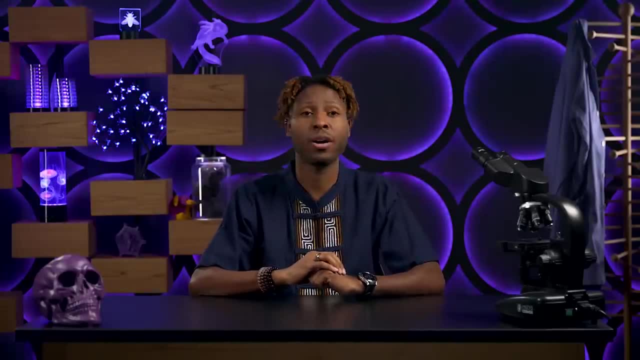 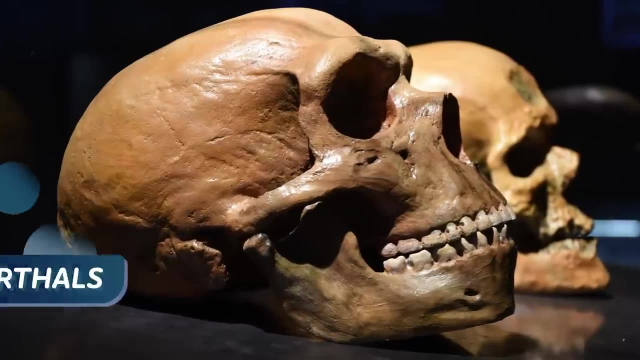 and they've learned that one part of the braided stream analogy is spot on. Ancient humans got busy making babies with other hominins as they spread across the globe. Our ancestors interbred with Neanderthals, some of our other hominin relatives who emerged around 400,000 years ago. 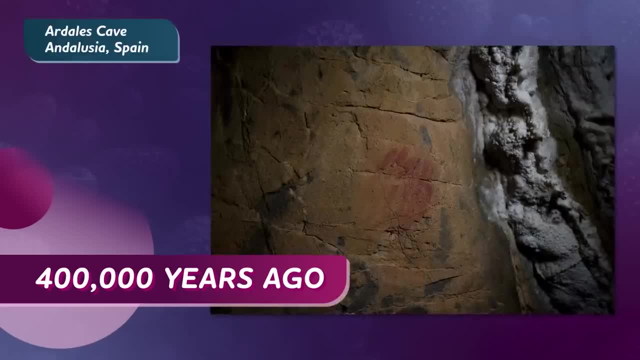 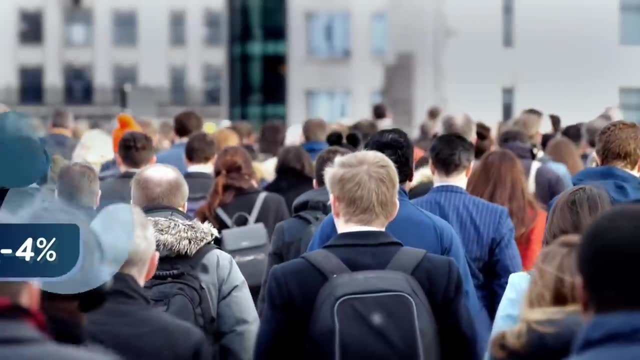 Much like us, Neanderthals buried their dead and made art. Because of those prehistoric relationships, many people today are walking around with a little Neanderthal in them — about 1 to 4% of their DNA. But are humans and Neanderthals the same species? 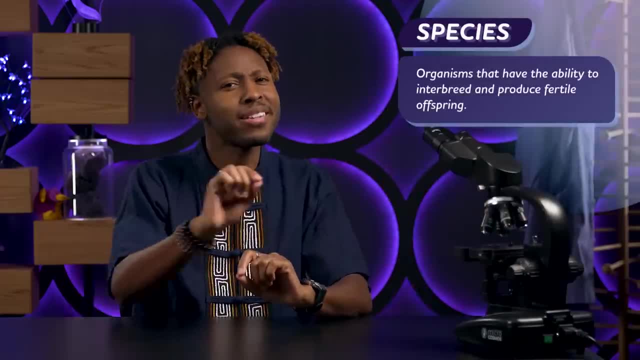 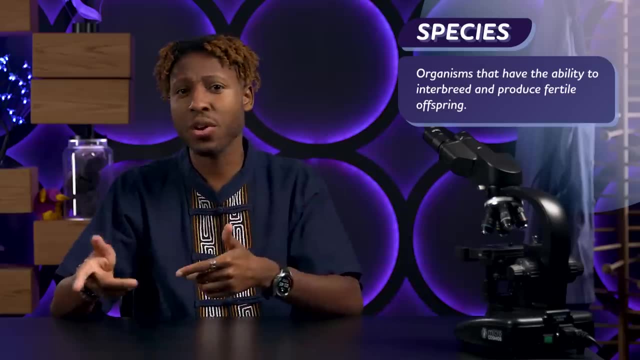 Well, not exactly. You see, some areas of science define species based on the ability to interbreed and produce fertile offspring, And by this definition you and Neanderthals seem like one and the same, But when scientists talk about fossils, we typically refer to Neanderthals as fossils. 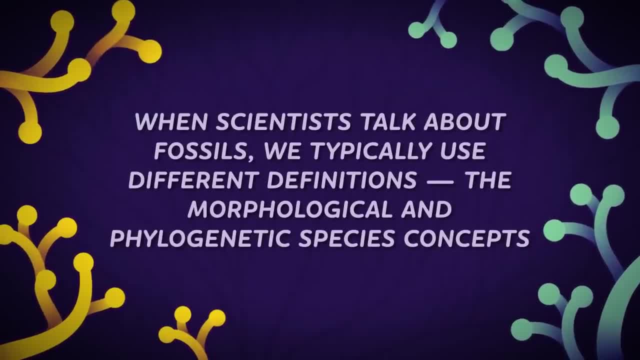 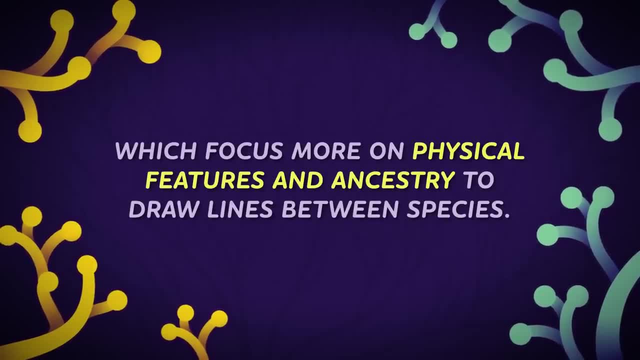 But when scientists talk about fossils, we typically refer to fossils as fossils. But when scientists talk about fossils, we typically refer to fossils. typically use different definitions: the morphological and phylogenetic species concept, which focuses more on physical features and ancestry to draw lines between species. 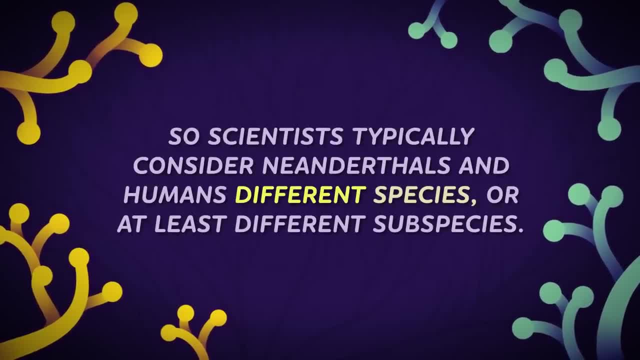 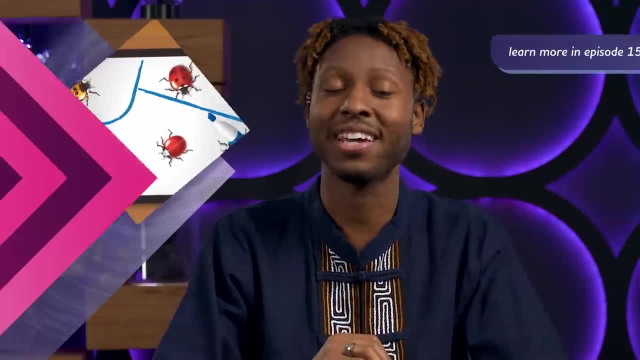 So scientists typically consider Neanderthals and humans different species, or at least different subspecies. You can learn way more about the trickiness of defining species boundaries in episode 15.. In any case, it wasn't only Neanderthals that caught our eye. 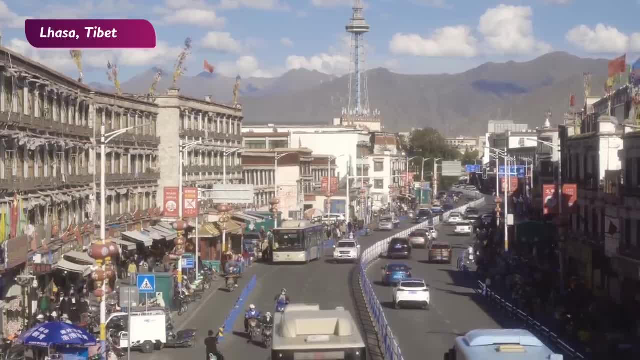 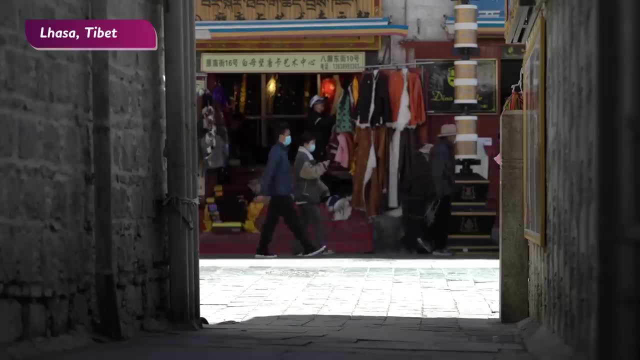 We also interbred with another of our ancient relatives, the high-altitude-adapted Denisovans, And because of that, some of us today are better at handling low-oxygen mountaintops, thanks to a genetic variant that came from that interbreeding. 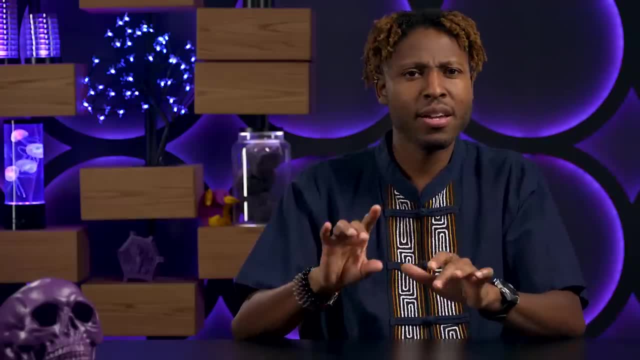 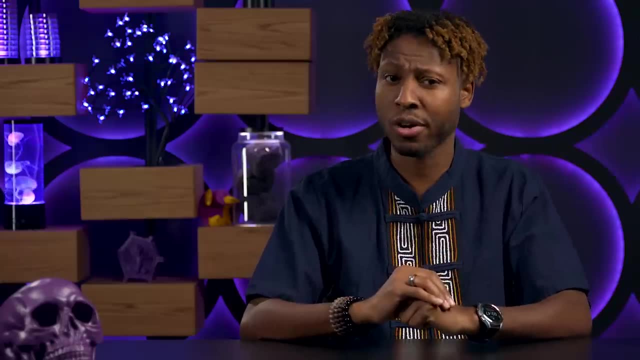 So the big hominin family tree, or stream, is one we're still wading through. Scientists connect the dots through fossils, genetic evidence and some major snooping on our ancient relatives, like three years deep into their Instagram at 2 am levels. of snooping And that helps us trace some of our ancient relatives. We also interbred with another of our ancient relatives, the high-altitude-adapted Denisovans. We also interbred with another of our ancient relatives, the high-altitude-adapted Denisovans. And that helps us trace some of our ancient relatives, the high-altitude-adapted Denisovans. We also interbred with another of our ancient relatives, the high-altitude-adapted Denisovans, And that helps us trace some of our ancient relatives, the high-altitude-adapted Denisovans. 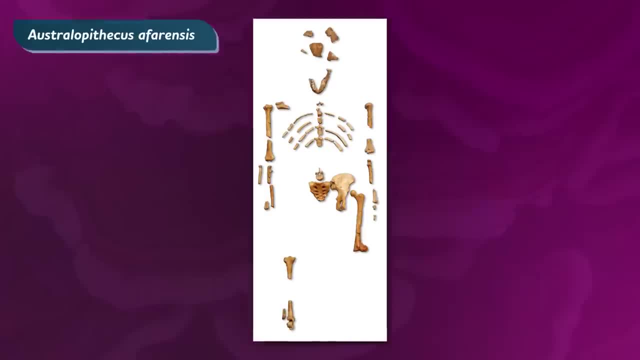 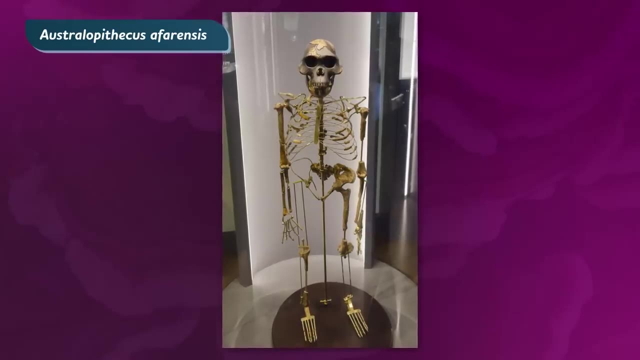 Some of the major leaps that we've made on our way to becoming human, Like remember our friend Graniapherensis, who walked around on two legs. Well, we know they got around that way. thanks to fossils and biological anthropology, We can see that the spinal cord passed through early hominin skulls, near the bottom rather. 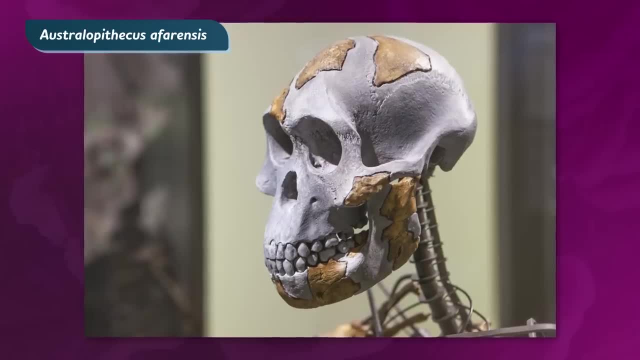 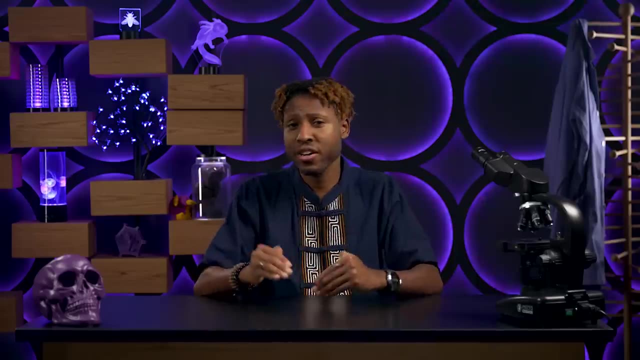 than the back, as it does with most apes. That means the hominin's head stacked above their body, a position that comes with walking on two feet rather than all fours. Walking on two feet freed up the front limbs, which we can tell happened before the invention. 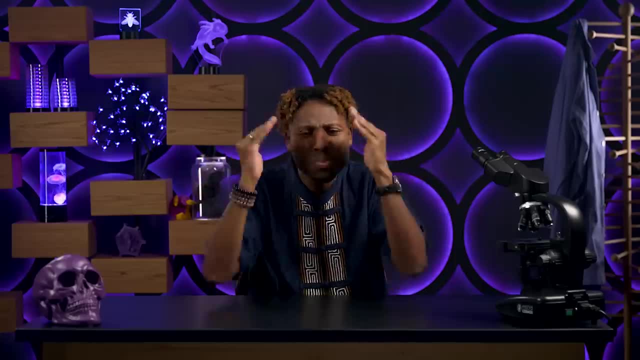 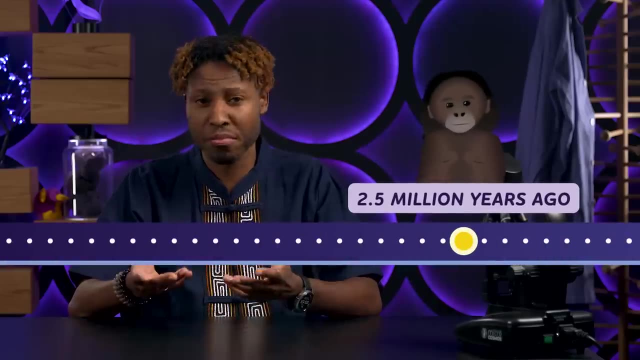 of photography, because what are we supposed to do with these on camera? Just… what, Anyway? by 2.5 million years ago, our ancestors were busying themselves with some early inventions, hammering rocks into tools that could slice meat off the bones of large animals. 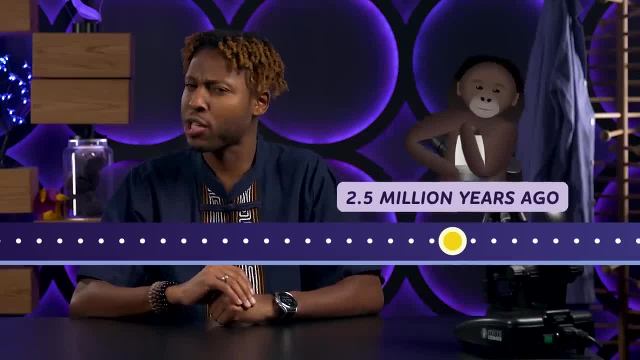 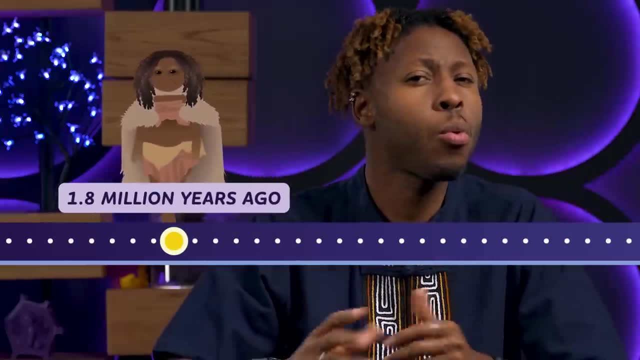 Think of it as the world's first kitchen gadget, the oldest ancestor of the slap chop By 1.8 million years ago. our ancestors had roughly the same body size and shape as we do, And they were walking long distances on two legs, like our friend Homo erectus, who migrated. 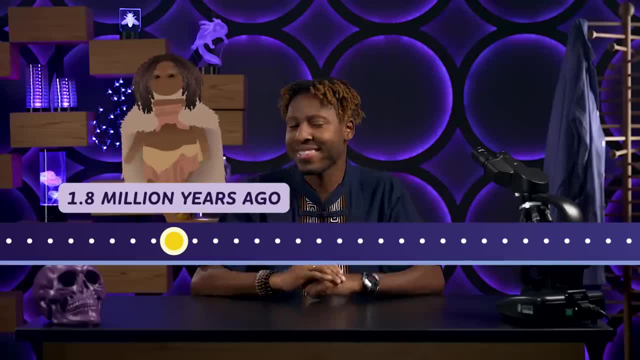 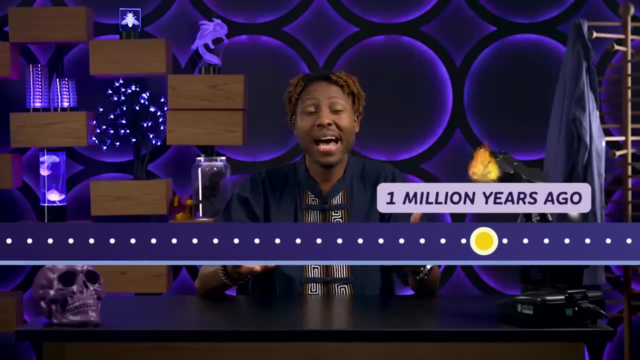 for the first time out of Africa, And as our relatives walked to new places, they faced new challenges and evolved bigger bodies and brains to cope with them. By about 1 million years ago, some of them had mastered fire, which we know from piles. 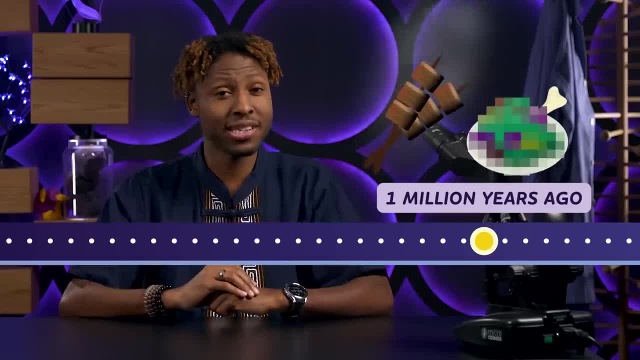 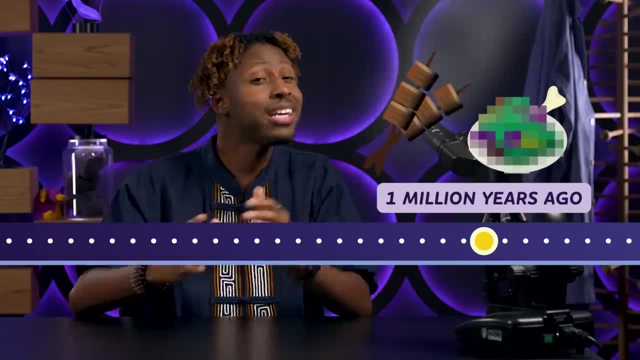 of ancient ash left behind in caves. With fire came the first attempts at cooking, which really makes you wonder why it took us so long to learn how to cook. It took us so long to invent chicken and waffles. if we had a million-year head start. 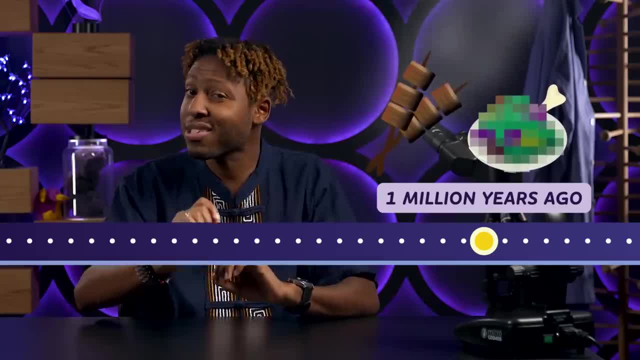 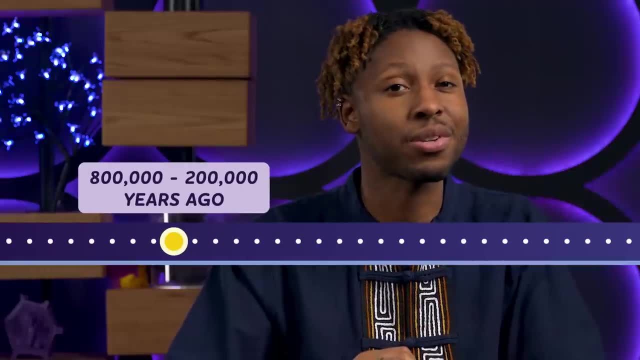 And even though they weren't cooking up soul food staples, their brains were steadily growing all this time. But things really picked up around 800,000 to 200,000 years ago, when our ancestors started communicating with symbols, sending messages with shared meanings. which might sound like 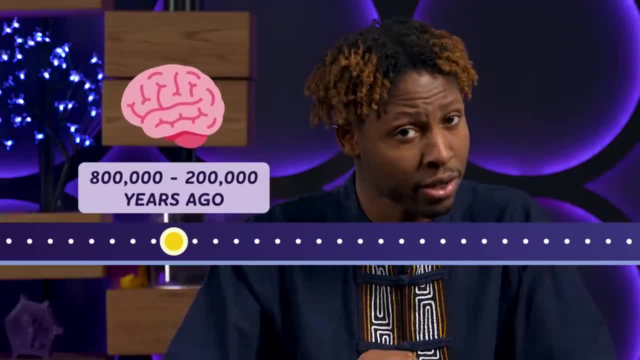 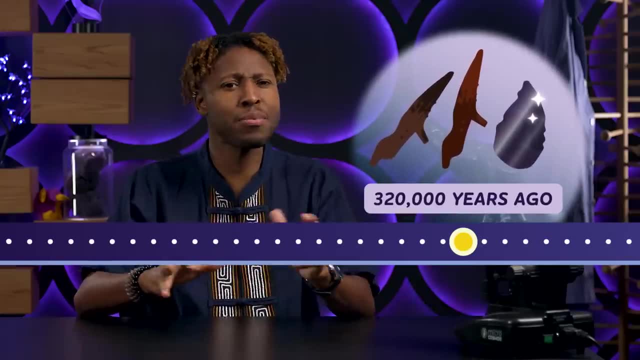 a no-brainer, but it was in fact a very big brain. As early as 320,000 years ago, they were fashioning red and black rocks on the surface of the earth. They even turned black rocks into crayons, possibly using them to decorate themselves. 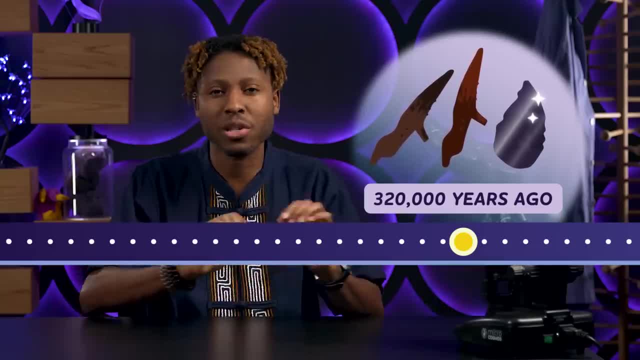 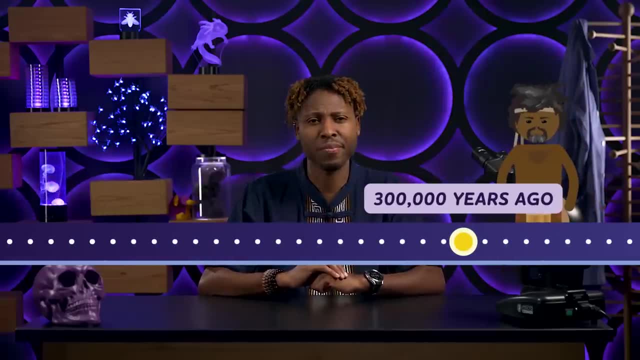 or their tools. They were also putting in the extra effort to transport special rocks over long distances. Modern humans finally arrived on the scene around 300,000 years ago. By then, our brains had tripled in size since the first hominin ancestors started walking. 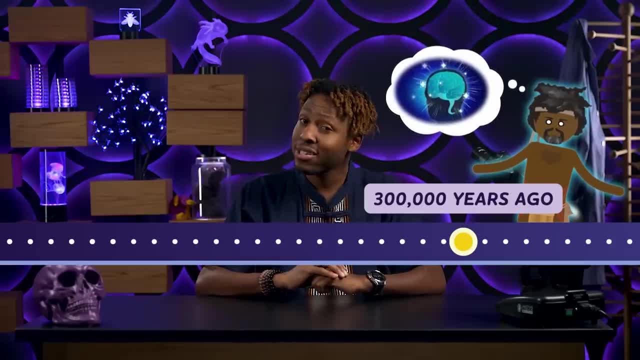 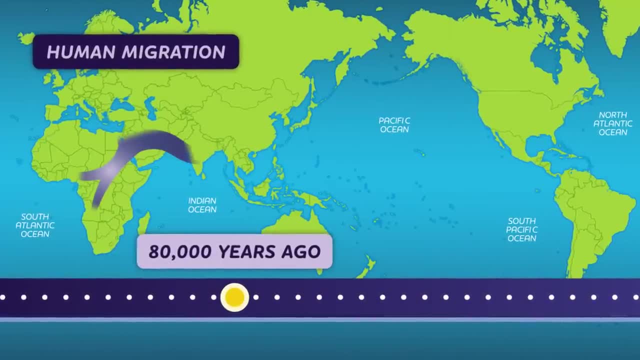 It's like the evolutionary biologist Stephen Jay Gould said: we stood up first and got smart later. By 80,000 years ago, some groups of wandering humans had migrated to other places like Africa and Africa, and migrated successfully across a number of continents. 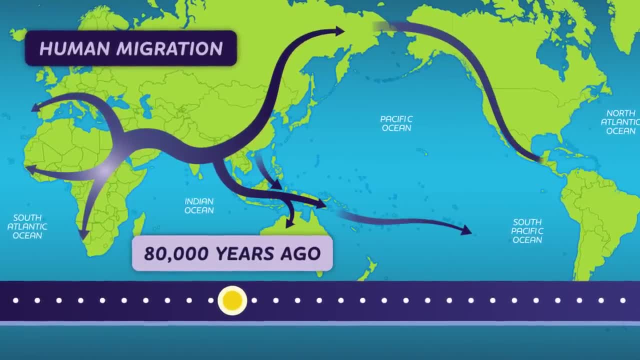 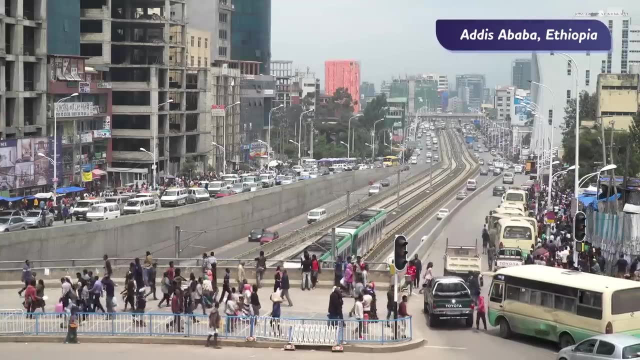 But each time a group struck out on their own, they eventually experienced the founder effect: a dwindling of their gene pool, which would lead to a loss of genetic diversity. That's why, to this day, people in sub-Saharan Africa are more genetically diverse than anywhere. else on Earth. It's because they're the descendants of all the people who stuck around, rather than smaller groups that moved away. At the same time, people kept moving and mingling, having babies with the locals everywhere they went, And that meant there was a lot of mixing between populations. 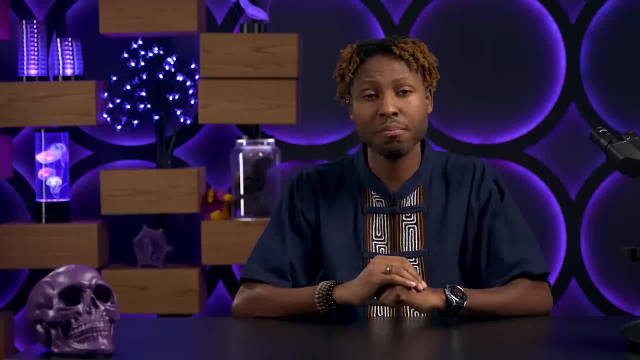 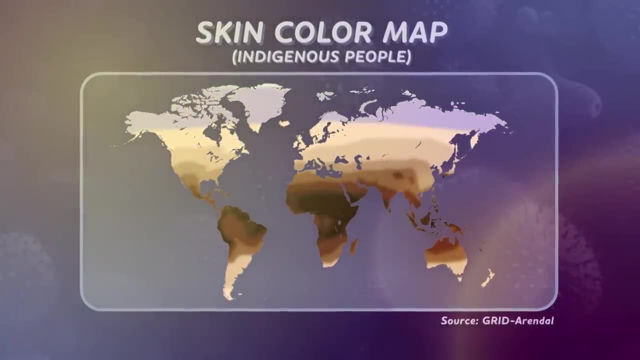 Even today, there aren't any hard and fast genetic boundaries between groups of people. As we spread across the globe, different traits evolved based on what helped our ancestors live and reproduce in different environments. The whole spectrum of human skin color arose to hit that sweet spot of blocking just enough. 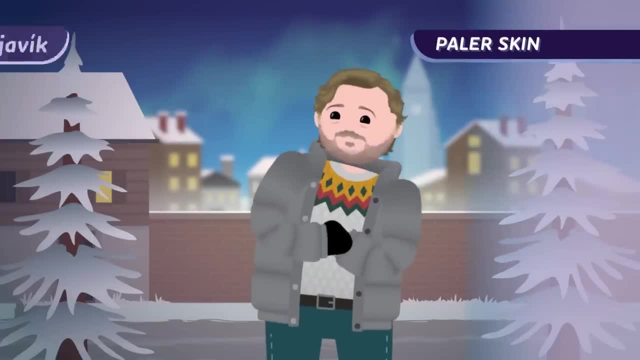 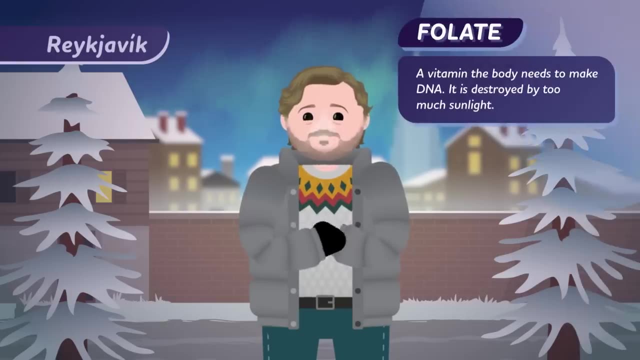 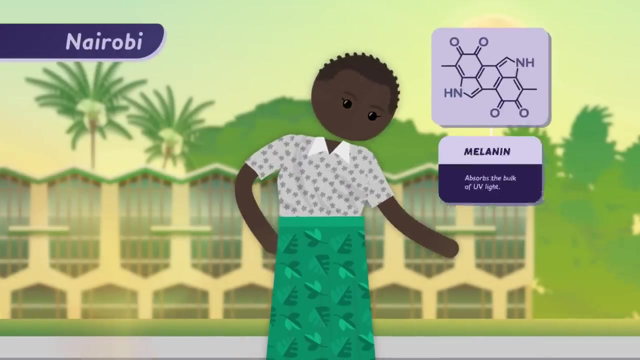 but not too much sunlight. People in less sunny regions evolved paler skin to allow for more UV absorption in order to produce enough vitamin D. Sunlight destroys folate, a vitamin your body needs to make DNA So closer to the sunny equator, people with more of the skin pigment melanin had an edge. 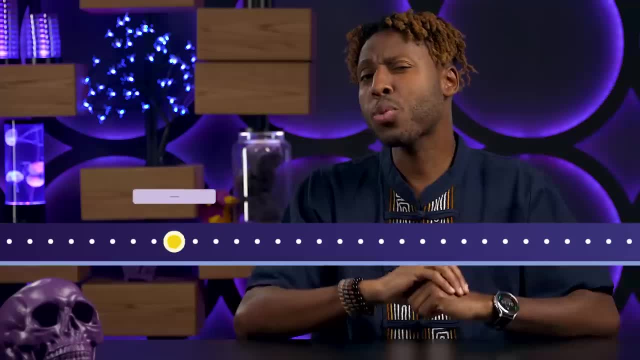 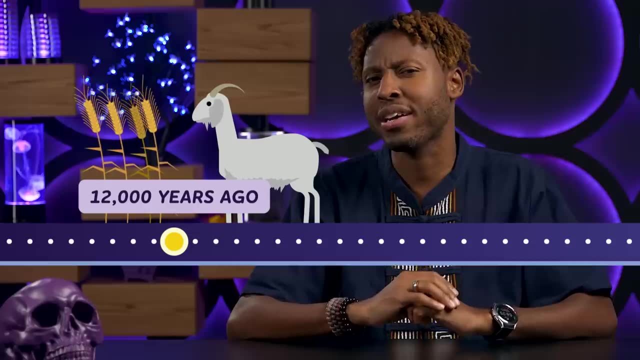 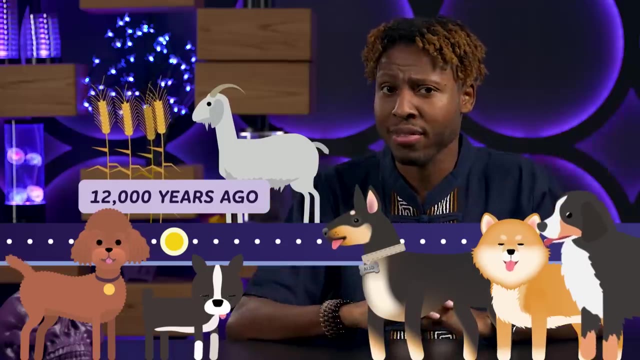 because of its ability to absorb excess UV radiation. Around 12,000 years ago, humans started domesticating wild plants and animals, selecting them for traits that we liked by controlling their breeding, That is, with one pretty big exception — dogs. We had already been hanging out with dogs for thousands of years by then. 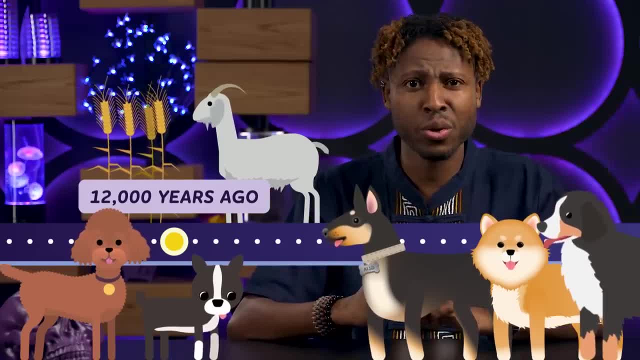 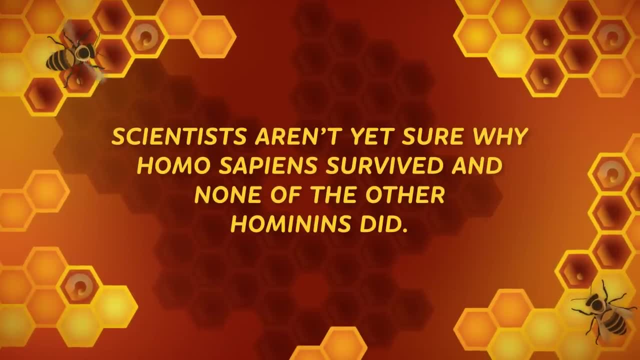 In fact, we've been pals with dogs for so long that it's not even clear who started it- us or them. And even today we're still evolving. Scientists aren't yet sure why Homo sapiens survived and none of the other hominins did. 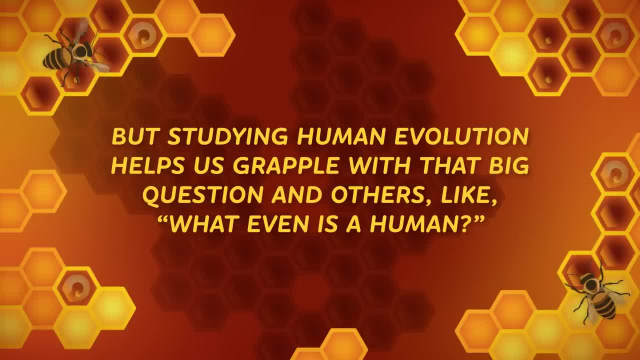 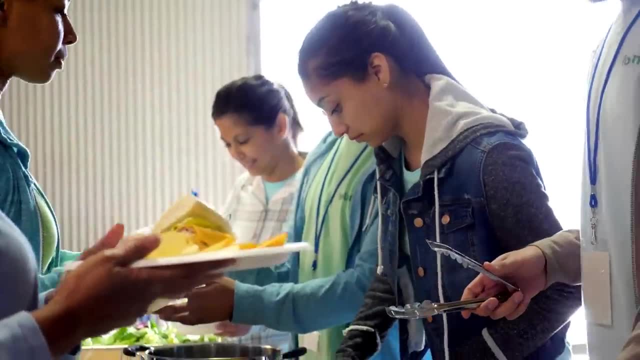 But studying human evolution helps us grapple with that big question And others, like: what even is a human? And while there's not one single answer, there are patterns, Sharing resources, caring for each other's kids and receiving care as we get older. 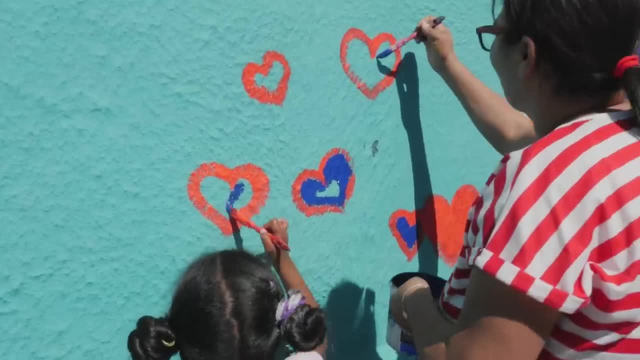 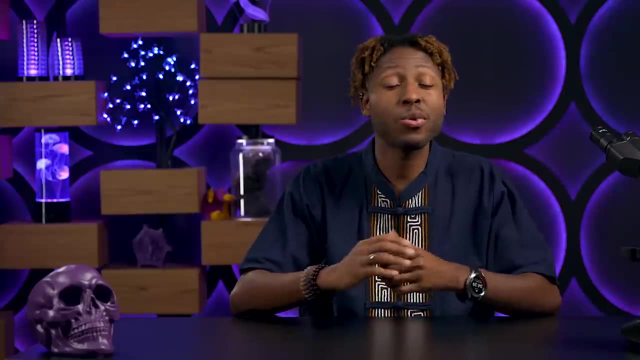 to name a few. Thus said, a lot of what we are as humans doesn't matter, It doesn't come pre-installed, We learn it together as we go. The more we learn from our ancestors, the better we understand ourselves. And by looking at our past we can imagine our future, not as a rigid, already charted. 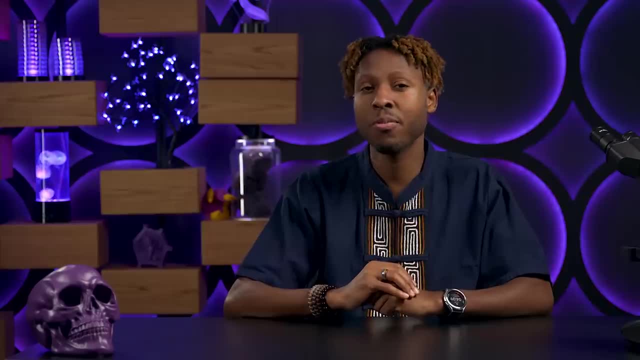 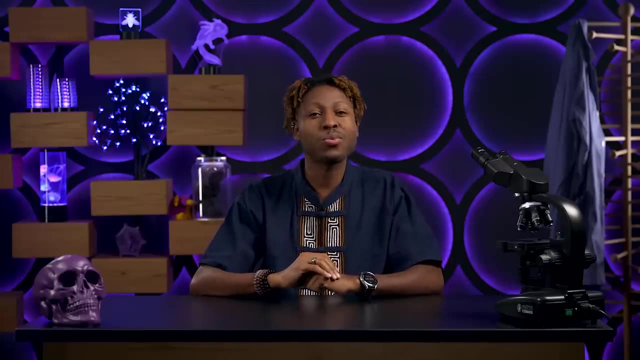 course, but as a winding stream that has been flowing for millennia And, with a little luck, we'll keep flowing for millennia to come. Join us back here for our next episode, as we move away from evolution and start talking about something equally as important, but physically smaller.